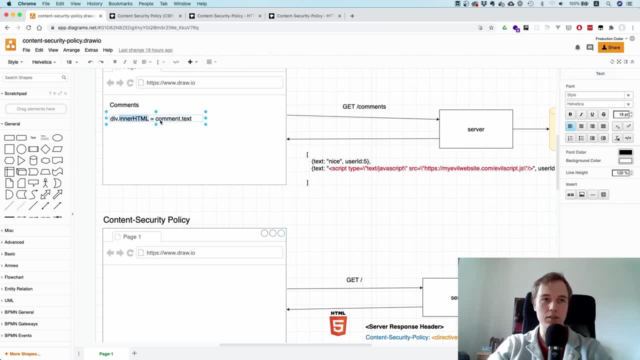 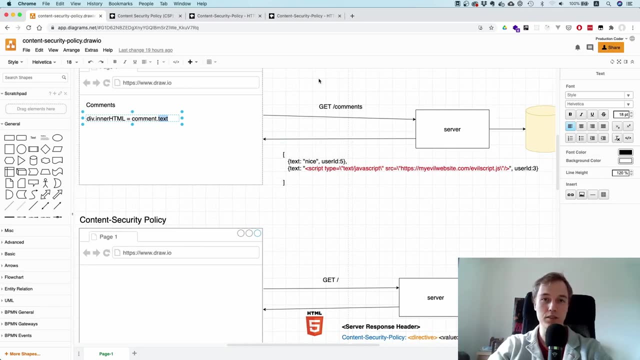 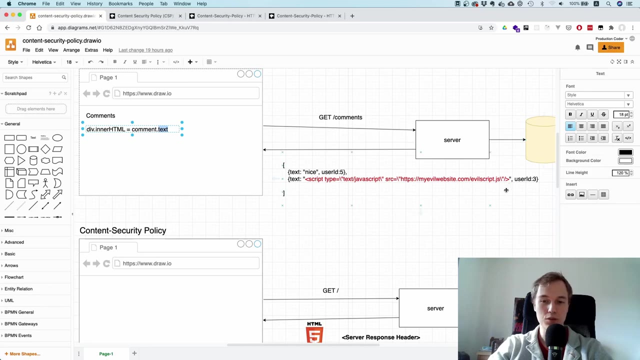 if you by accident say, okay, the inner html of this div is the text, and you just say, oh yeah, people are just going to put the text, then you have a big security vulnerability, because what this means is that once this comment here is posted and stored in the database, everyone who's 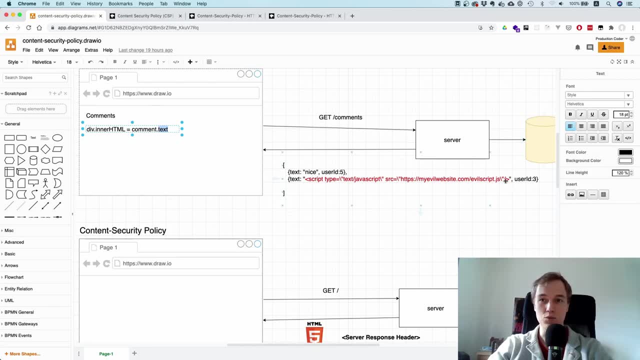 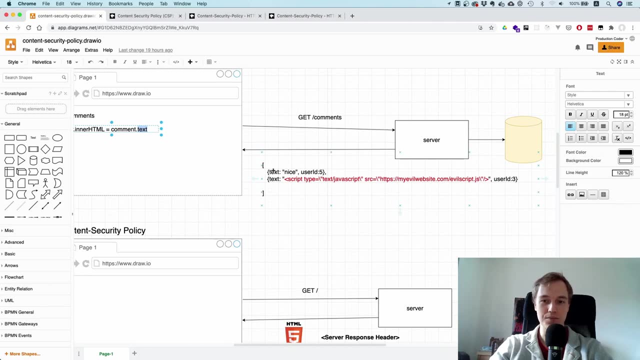 going to scroll through the comments after that will have this additional html tag in your website and all of a sudden, everyone who is watching this video, everyone who gets on that page, the browser will just load, like this script from this origin and the script will execute evil- uh, do evil things. 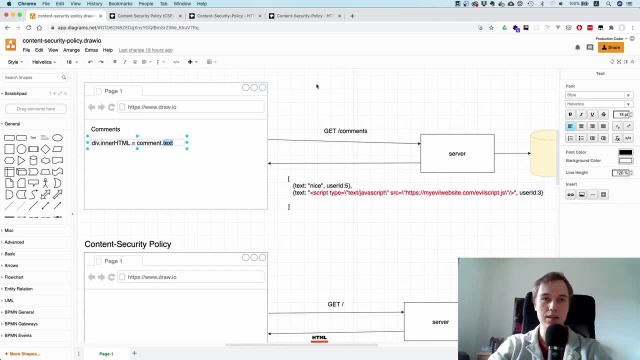 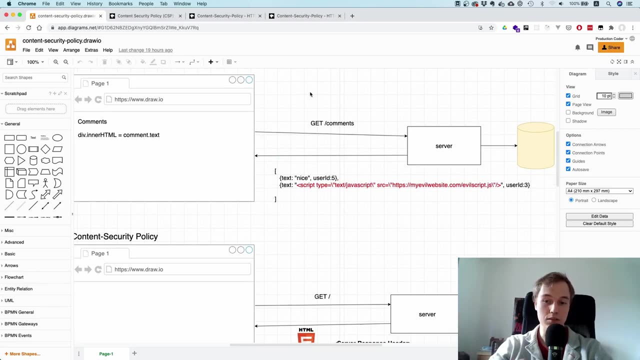 and that's why this thing is called a cross-site scripting. so basically, the idea is that some attacker is able to inject some script into another person's browser, or they have a script that they want to use, and the attacker can do so by exploiting the belief that everything. 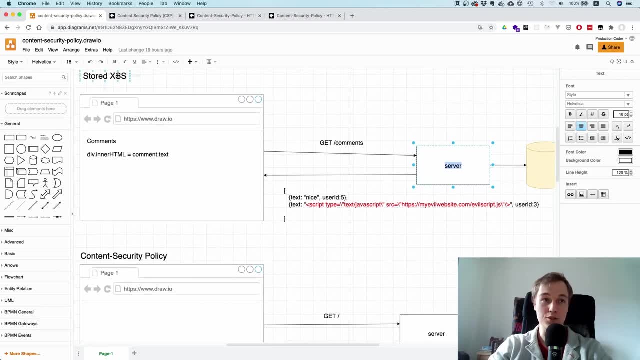 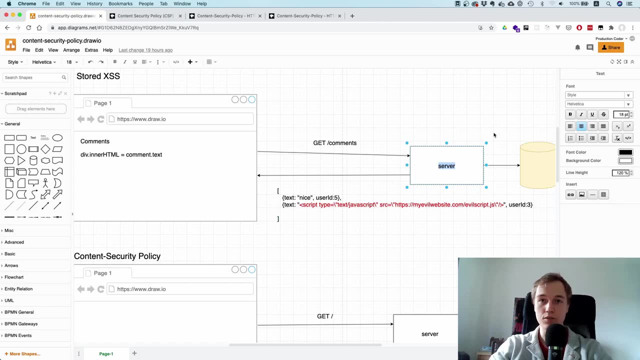 that comes from your own server is kind of safe, and what i've just shown here is a special type of cross-site scripting which is called the stored cross-site scripting, simply because the attack is actually stored in the database. so there's also other types of cross-site scripting, uh, reflected. 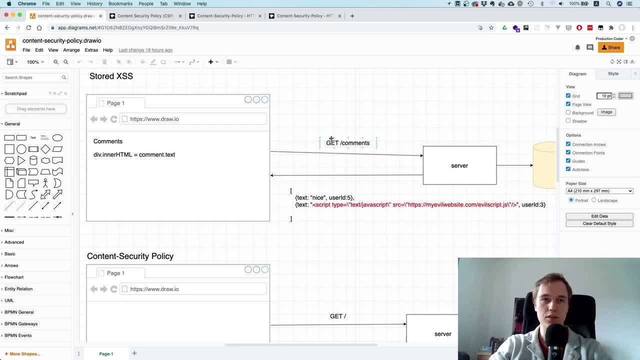 cross-site scripting, dom-based cross-site scripting, but i think this one is like the easiest variant to understand. okay, and what we want to do with content security policy. we want to protect ourself against this and the idea here is that we just come up with a policy and that tells the browser. 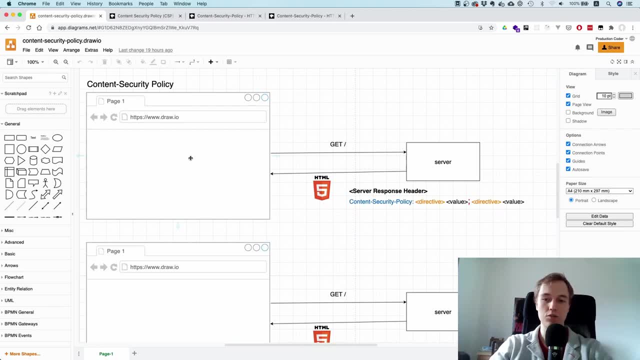 look, no matter what happens, you're only allowed to load script from this origin, this origin or this origin, and you're only allowed to load images from that url or this origin and the other origin, and you're only allowed to load fonts from here, here and here, and that is the main idea. 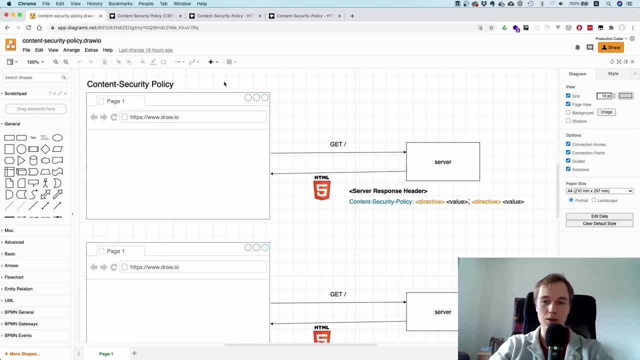 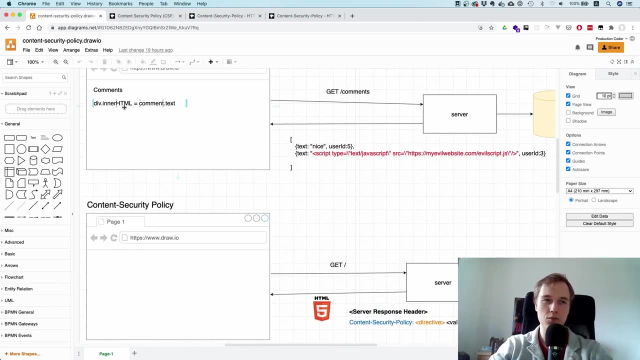 of the content security policy. so you basically hard code which from which origins you kind of expect to load content. and even if something like this happens- so even if you make a mistake here and you know you just forget about it, even if that happens you will not. 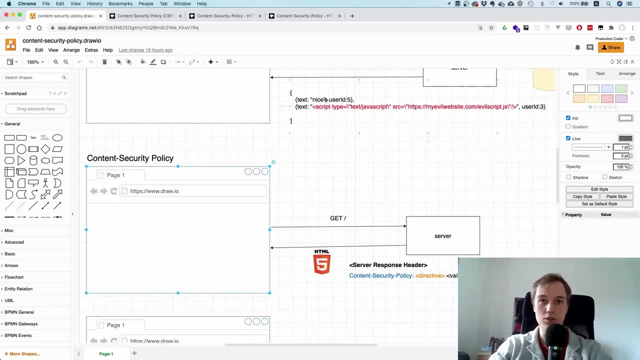 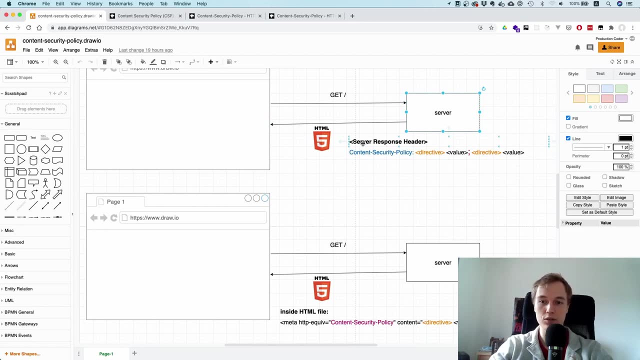 have issues. if you have like a proper content security policy, the browser would just block this script, so it would not load it. the way this works is you can just return an additional header in your server response. so that means once the person goes to the website and the html. 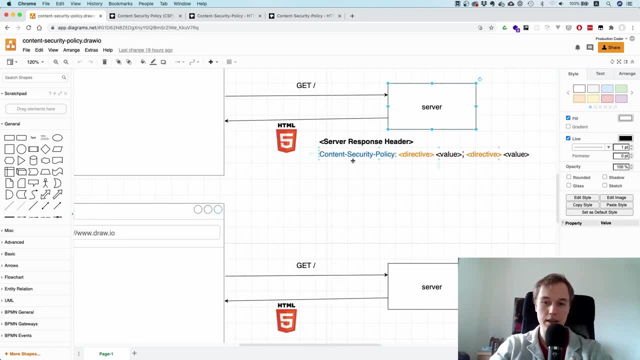 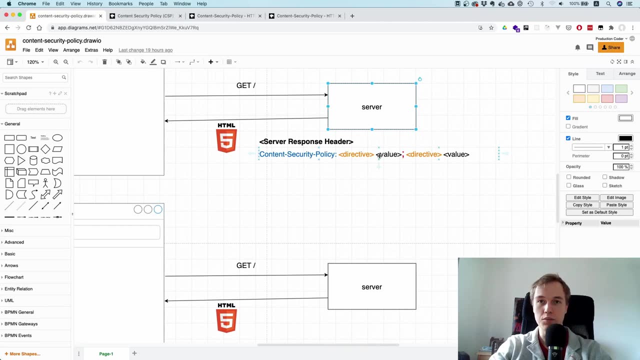 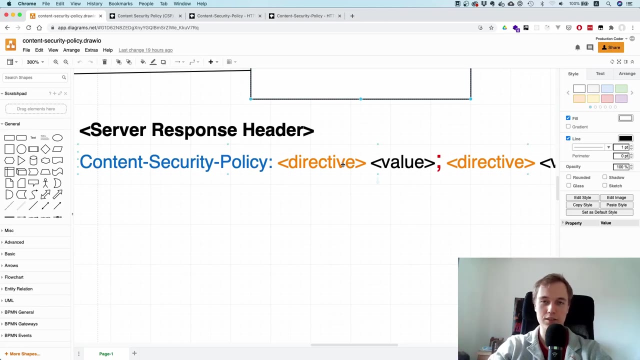 file is sent back, you just add like an additional header, and that header is called the content security policy. inside of this policy you have directives and you have values, and the important thing i want to make clear here is that it's not key colon value, basically the default syntax in javascript, but it's just the key, so to say, the directive space. 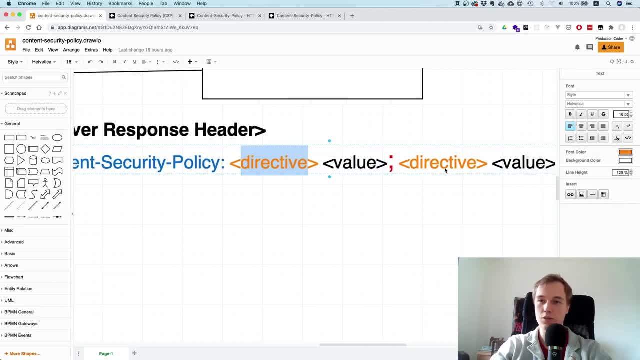 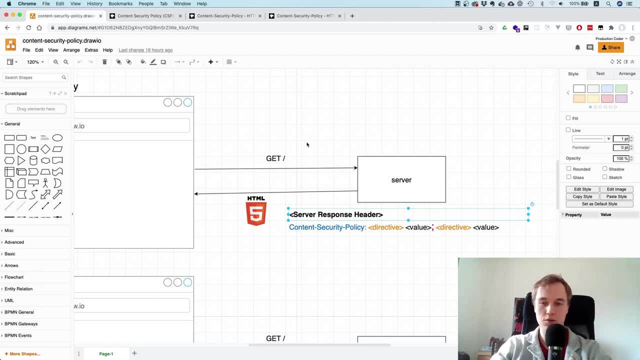 and then the value, and then you have a semi-colon and then you can have the next directive. as long as your server has like this header, you're pretty well protected against scripting, So that's pretty good. And another thing I wanted to mention is that you can also 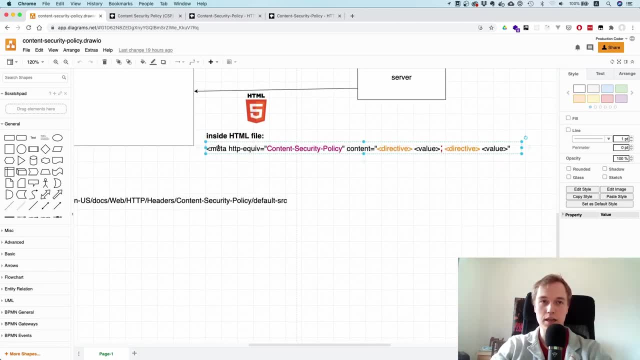 put this inside of the HTML file by using this meta tag, So you can say, hey, here's like some metadata and the HTTP like equivalent is the content security policy, And then you put the string inside of like the content property And yeah, this is like how this works. So, hopefully, 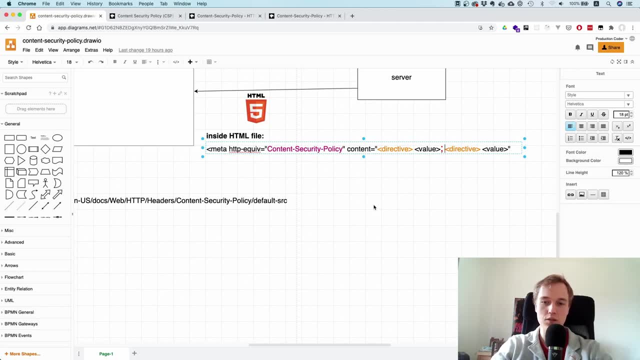 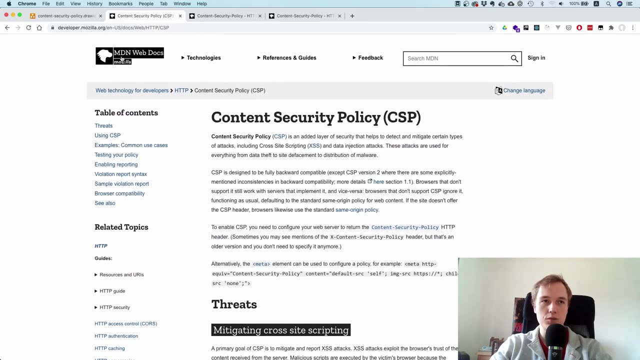 this is this? now made clear what the purpose of content security policy is, And let's just take a look at the documentation. So I would recommend you go through this MDN web docs. I think it explains really well what it is. So, with the explanation I just gave, I think it's this page. 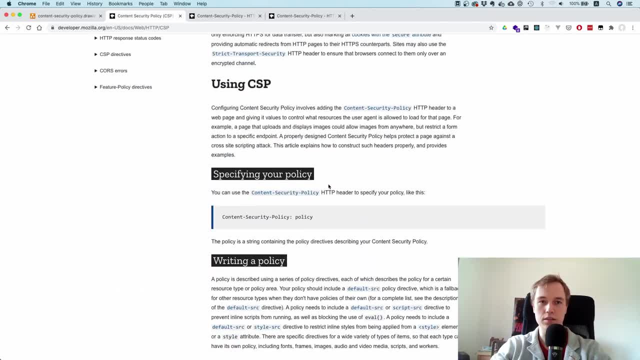 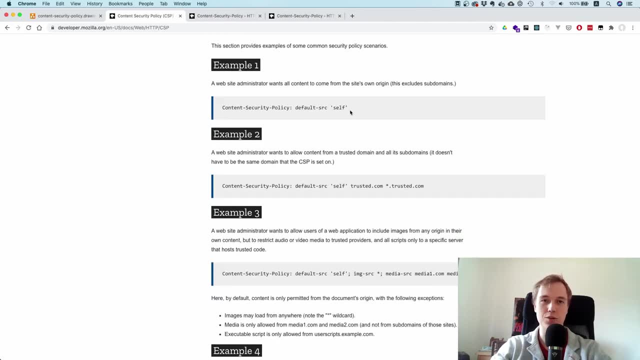 is way easier to understand Now. you can scroll through all of this And you know there's also a couple of examples over here, And these examples are very useful because you just see what's going on. So, for example here, this is, I think, also important to understand. what is this default? 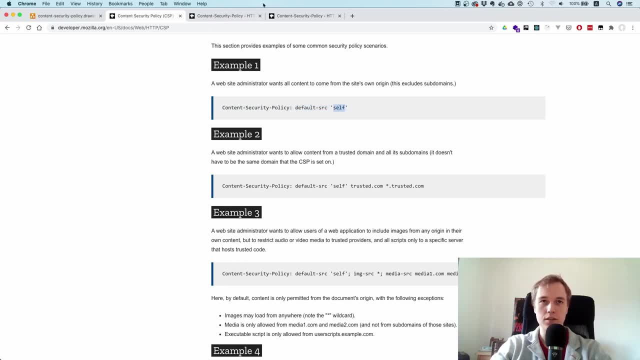 source And what is the self. So the thing is, the content security policy allows or gives you very fine grained control. So you can say: I only want to load fonts from this origin and I allow scripts from this origin and I'll. 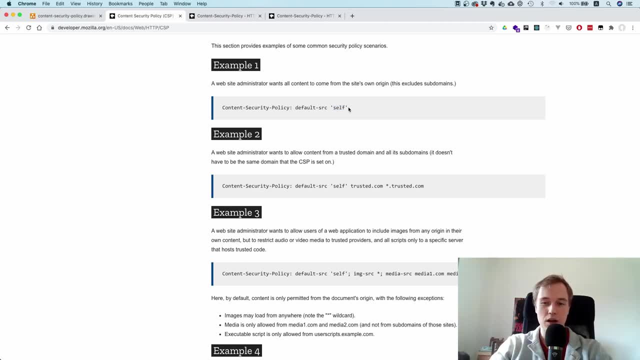 allow images from this origin and so on. Sometimes people are not, you know, that specific And in that case this default source kicks in. So think of, like, if you think of a switch case statement, this is like the default clause, right? So if there's nothing specified, 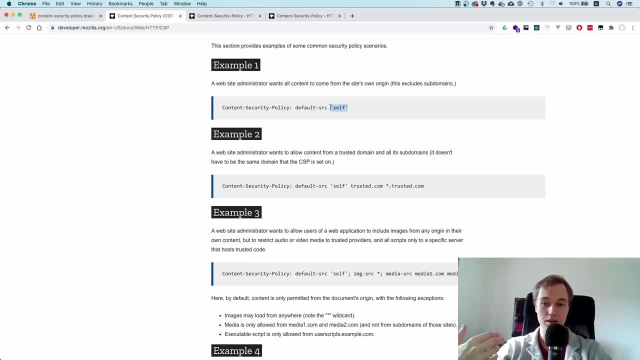 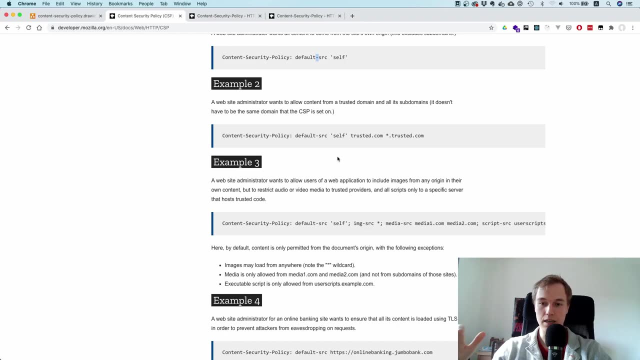 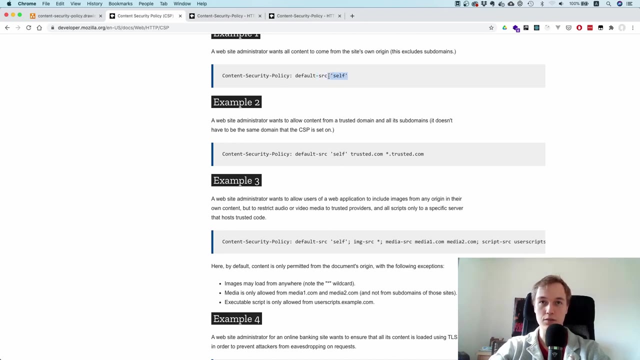 it will just say self, And self means like your own origin. So that means if you don't explicitly like, specify that this URL, that we can load like fonts from this URL, then the default source will be self, which will mean if you attempt to load like the font from another URL, it's going to be. 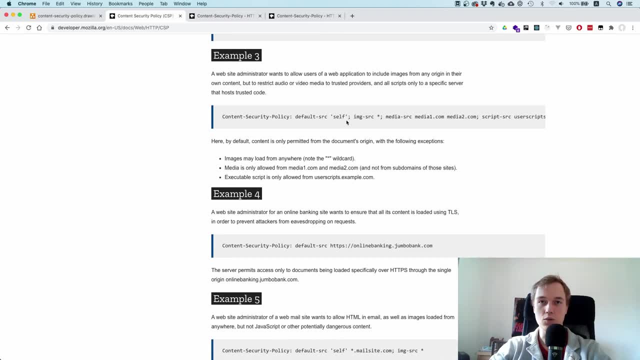 blocked And you can. you can see like more sophisticated examples here. right, you can see like media sources and these types of things. So, if you want to load fonts from this URL, you can see like more sophisticated examples here. right, you can see like media sources and these type of things. 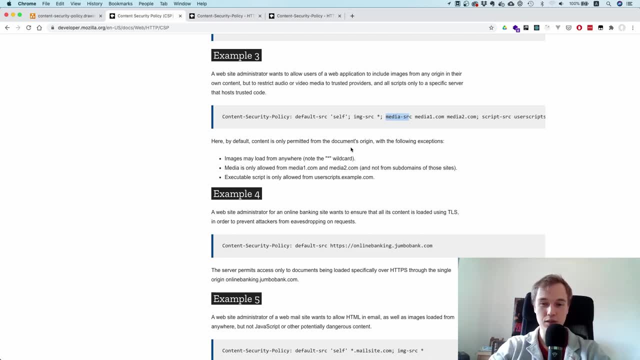 things. I'm not going to go through all of these directives. I also don't think you need to learn them by heart. I think you just need to know what it is And then you can, like systematically and step by step, develop your own policy. And what I would also recommend is that you go over here and 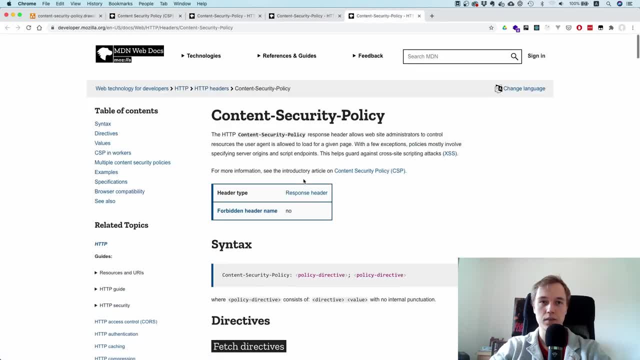 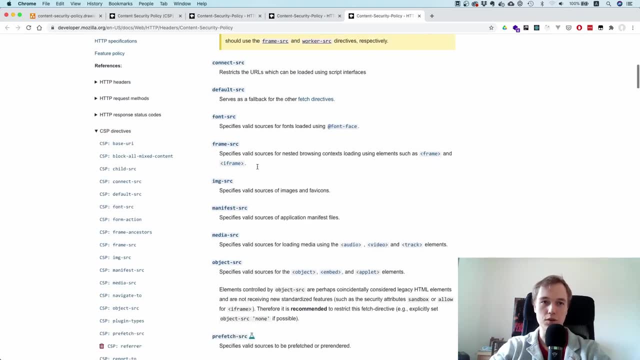 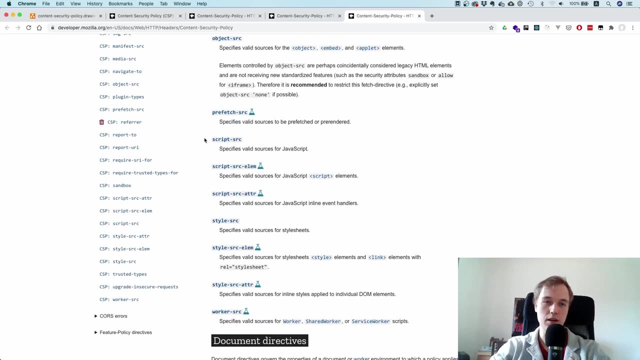 click on this Because here you can see like here it explains like all the different directives. you can have the thing I just mentioned: where can I load fonts from, Where can I load images from, Where can I load like objects from, and so on and so on. So you can see here: yeah, script source as: 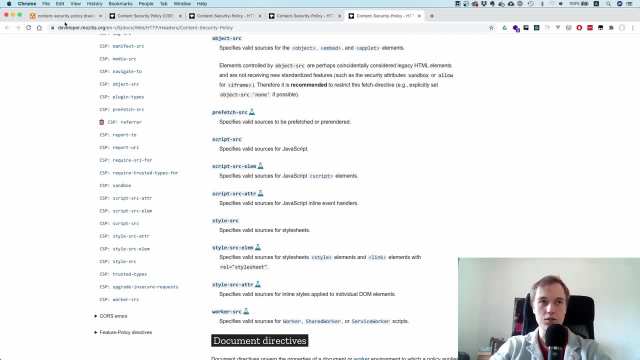 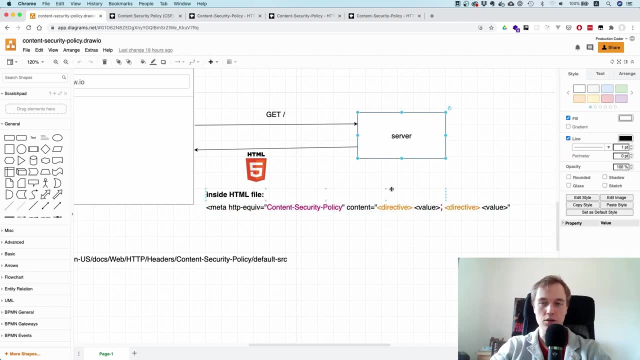 well, So these are the directives that exist, And the question is now is what does that mean for you in practice? So in practice, this means, if you have a server or if you have any type of like website or front end, that you return to the browser, regardless of whether you're doing. 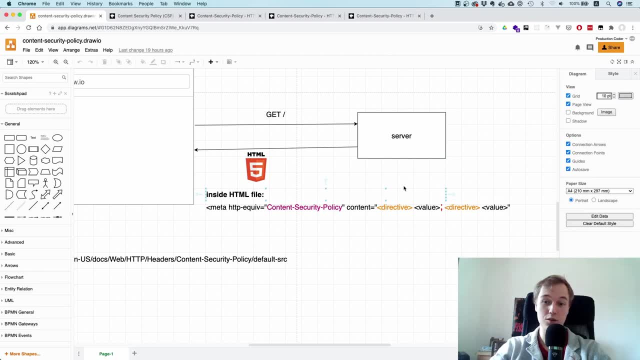 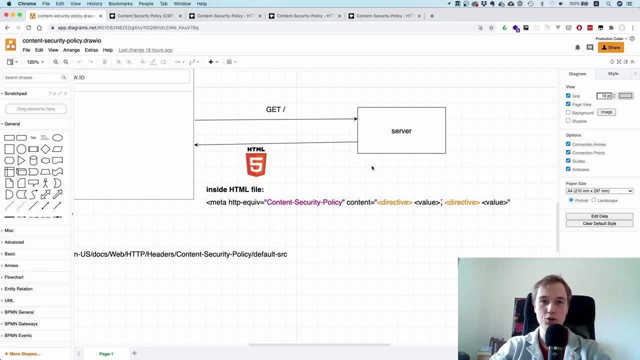 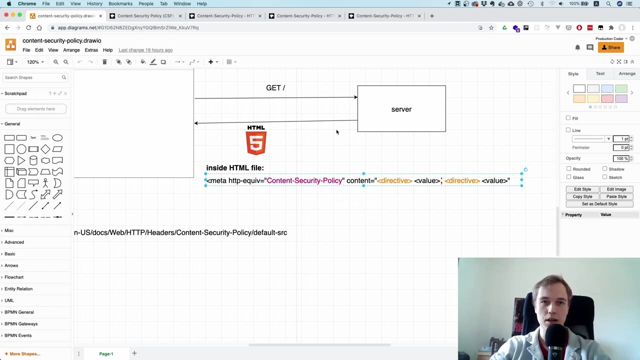 server side rendering or whether you use, you know, whether you have a single page application and you make like cross origin requests to like an API gateway later on, you should always include this header like this meta HTML tag, because if you do, you are just very well protected against these stored and 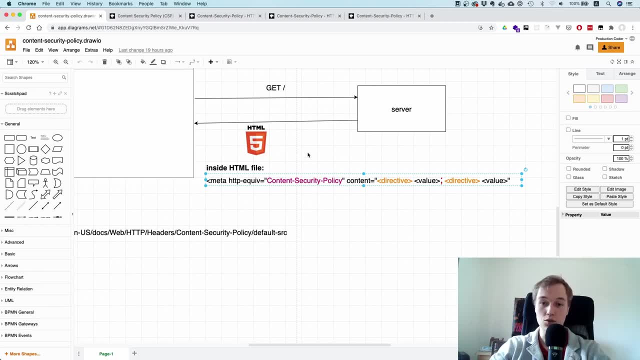 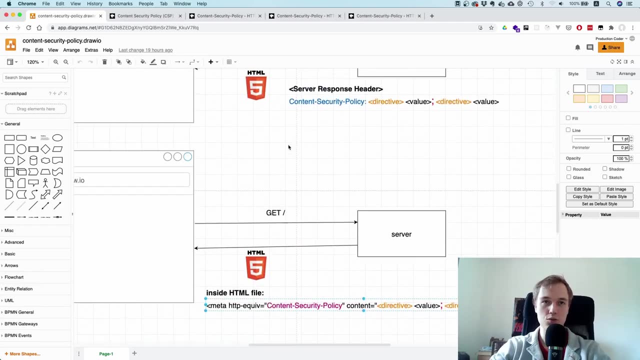 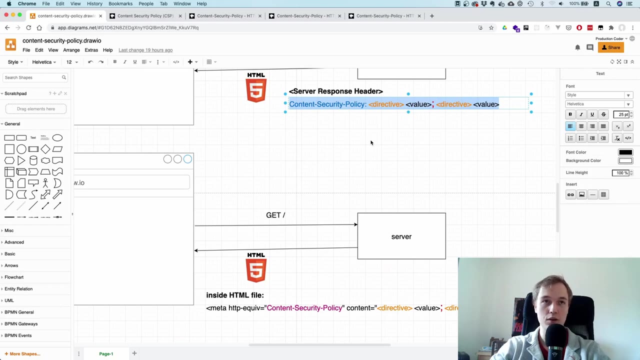 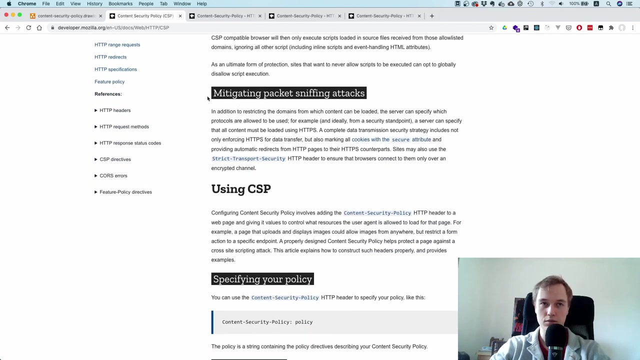 reflected cross site scripting attacks. Yeah, so make sure that if you deploy whatever you want to deploy, your react to Vuejs app- that you have some sort of content security policy and then you can mitigate most types of content of cross site scripting attacks. Yeah, another thing I just forgot to mention is that it also like the content.